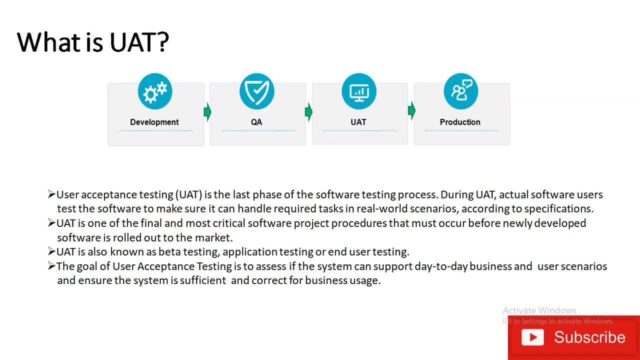 before newly developed software is rolled out to the market. So UAT is also known as beta testing, application testing or end user testing. So after completing UAT testing, the software user must be able to access the software and the software network roku the development and the testing phases. UAT introduced at the end of the 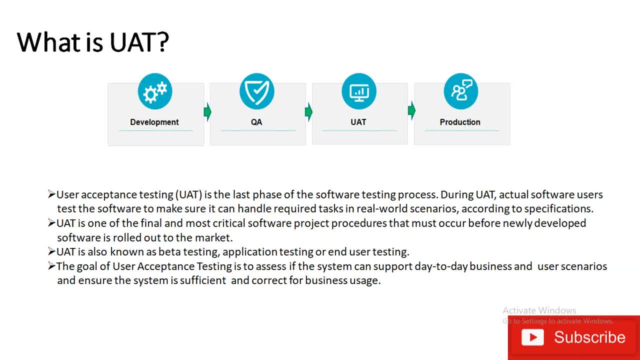 testing. So if you uefi testing is done by who has provided or who wants this application to be delivered to the end user. The goal of user acceptance testing is to access if the system can support day to day business and user scenarios and ensure that system is sufficient and correct for business usage. 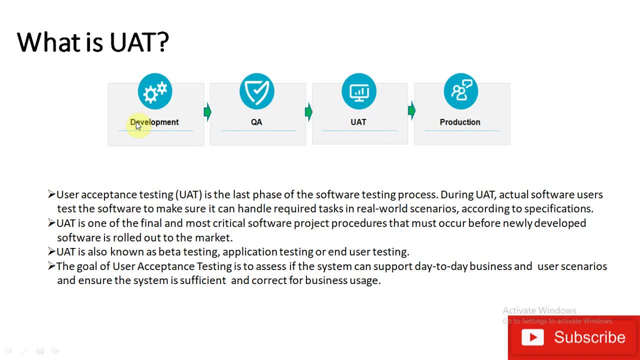 So, as you can see in this image, there is a development. So development team will create that application based on a requirement which is shared at the initial phases of the application process. Then, after development, they will provide that application to the QA team and QA team certify each and every steps. 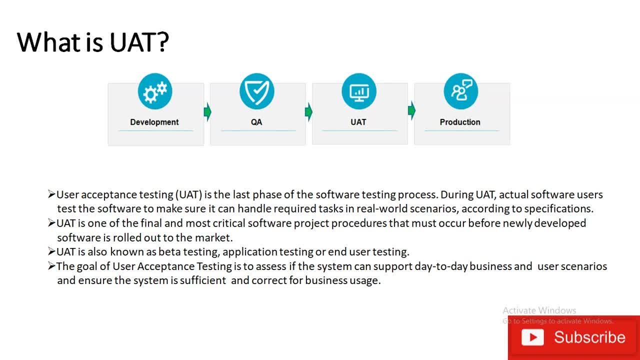 and once QA team certify and deliver to the UAT, the UAT team should test that application based on their requirement. So the question is: is that application is built based on the requirement, is functionality is massive or end user is happy with that application? 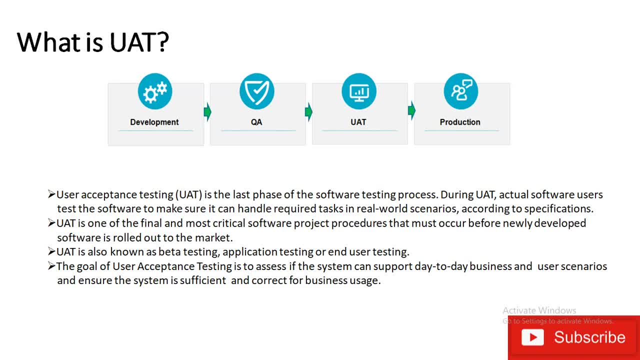 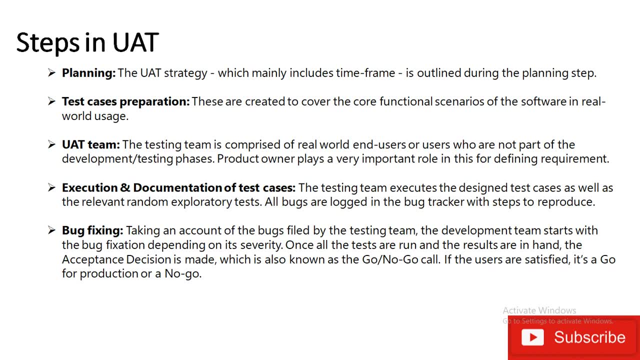 Then it moves to the production phase. So this is all about the process from start to end. So what all steps or phases is involved in UAT? So first is planning phase. So in the planning phase the UAT strategy, which mainly includes timeframe, is outlined. 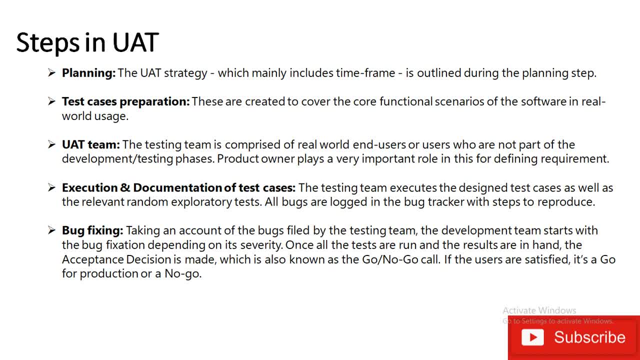 during the planning phases. So in this phase the UAT team will plan accordingly how we can test that application with the test cases and what all functionalities are included which all applications require to test that that application or the product which they have received. 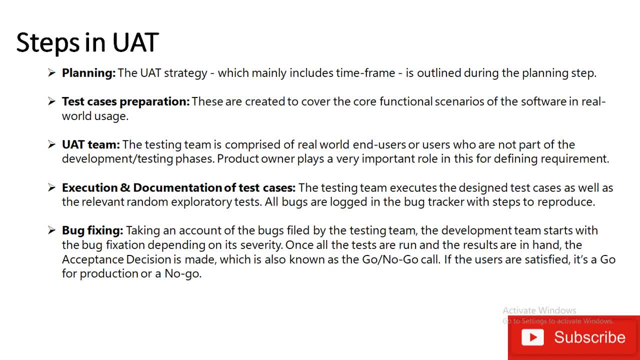 So it also includes their environment, setup, application needed, resources needed, how much time it will take to complete the UAT testing. So these all are requirement at the initial stage we test that UAT phases or before starting in testing, so that should be planned accordingly before starting the. 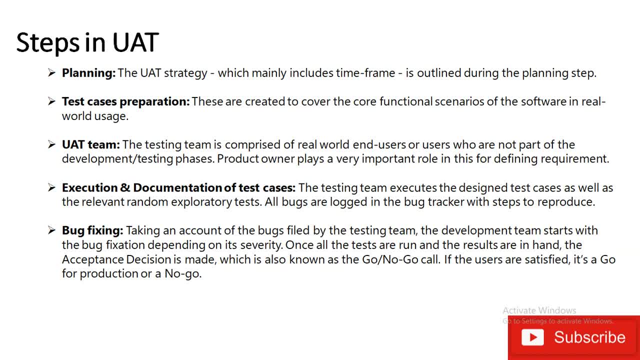 uat testing. so next next is test cases preparation. so these are created to cover the core functional scenarios of the software in real world usage. so test cases preparation will be done based on the requirement and input received from the product owner or by the owner who wants this application. 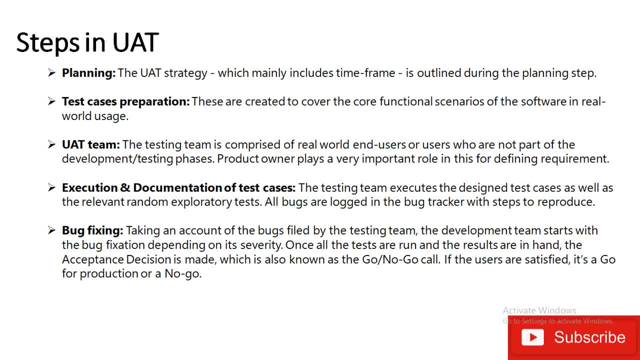 to be delivered in production. so test cases are mainly on the functionality part. then the performance is also a part of a testing. so load, stress and and performance should be covered in uat testing. so these all cases should be prepared in test case preparation and that is sign off by the product owner. so for those who are looking for performance testing, 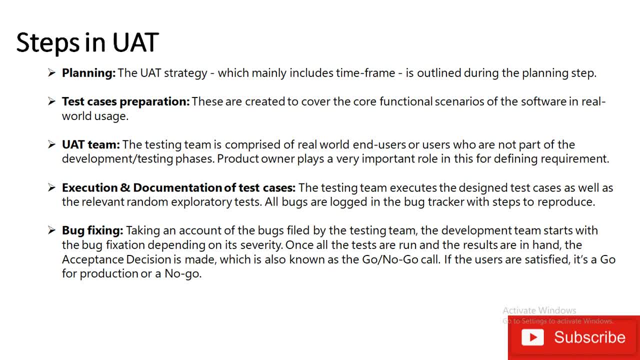 art session or load testing or these i have already covered in functional and non-functional testing. please watch that first, then you will understand that concept. then next is uat team. that testing team is comprised of real world end users or users who are not part of the development or testing phases. 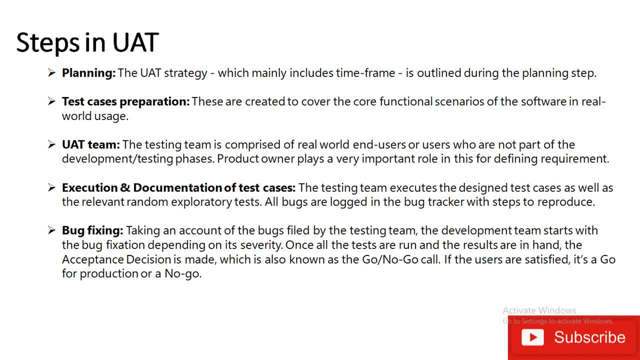 product owners plays a very important role in this for defining the requirement. so uat team is comprises is basically they: uh, the team is also called as beta testers or alpha testers or gamma testers. so all these are requirements are done in the uat team so that application is going to. 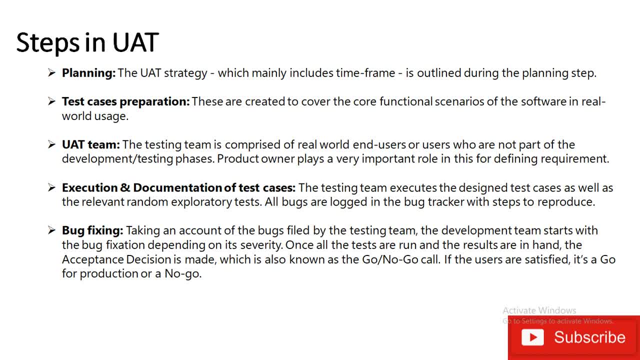 implement or it is going to beμά easy um of the application. before that they have to certify the application is exact or to the mark of the application. then next weeks, execution and documentation of test cases. so whatever they have and created the test cases by the uat team and based on their preparations, they will execute that. cases and after acquisition, they will create a uatt application. you know that virtual test cases are built a t versus false. I have been outside our intention to talk about a serbs review, so let's quote out, for example, the uaty team then and uh post. but they have done by our own company contract as per actual test time, which, of course, is only 58 hour per day and basically each test case the tools of yo and i are required by. if each sub is displayed on�� clamline and android, testimony materials will be supported and entered into test next step, which is the application. now, if you think this video is complicated by this, 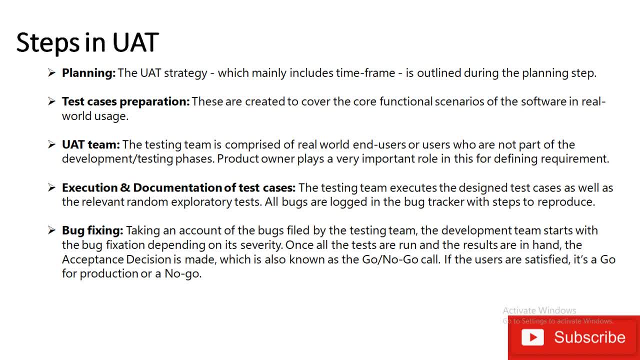 a execution report. then if they found any defect, that defect is locked or send it to the developer team and developer will fix that defect. after fixing they will again retest that application and do the regression for that and then only they will provide go or no go. so, taking account of the 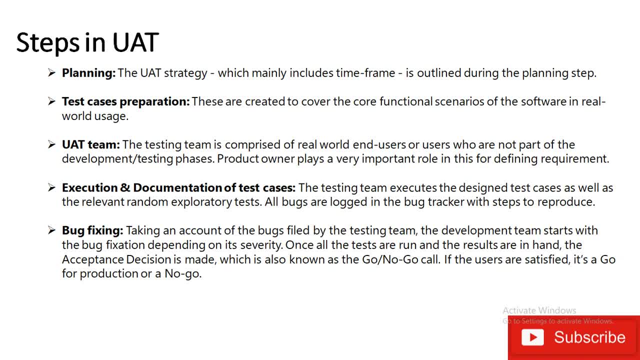 bug field by the testing team. the development team starts with the bug suggestion, depending on its severity. once all the test cases run and the results are in hand, the acceptance decision is made, which is also known as co or no go call. if the users are satisfied, it's a go for production. 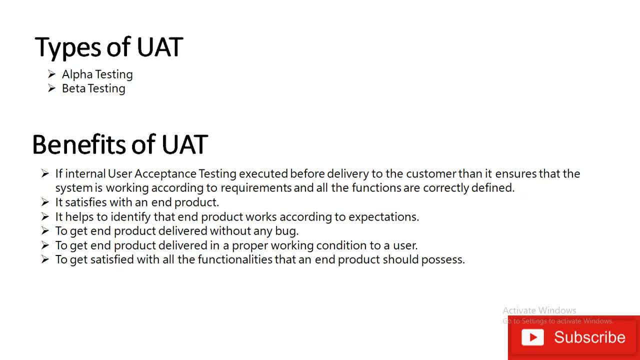 or a no go. so what? all types of the uad testing will be done. alpha and beta testing is majorly a part of the user acceptance testing. for those who are looking the complete session on the alpha and beta testing, please watch my previous session on alpha testing and beta testing. i have already explained about alpha. 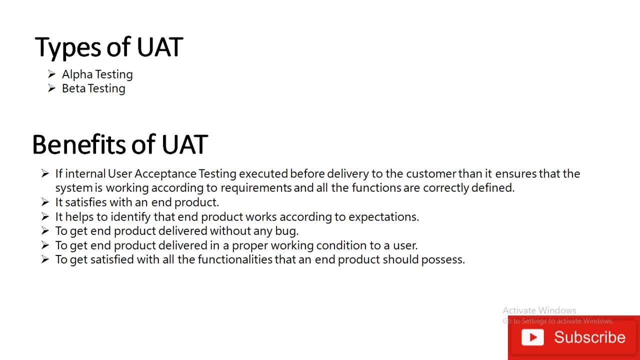 and beta testing. here i am covering only user acceptance testing. so what all benefits we will get while doing user acceptance testing? if internal user acceptance testing executed before then it ensures that the system is working according to our requirements and all the functions are correctly defined. it's satisfied with an end product. it has to identify that end. 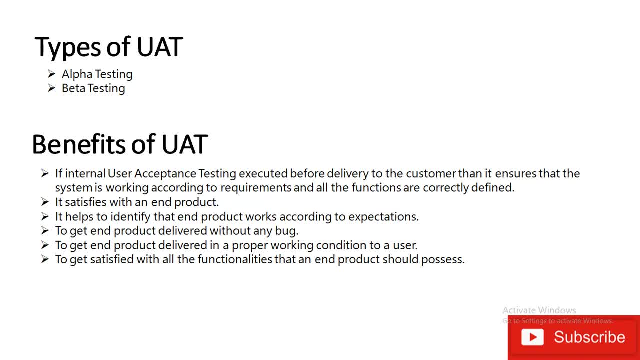 product work according to expectations. so if we are talking an example of whatsapp application and the owner wants to create video calling, and if that video calling feature is not available in the whatsapp application and successfullyoganize the developer testing wonder team, then the hormones oil clap and checking cd value and Yo Ken Mansha. 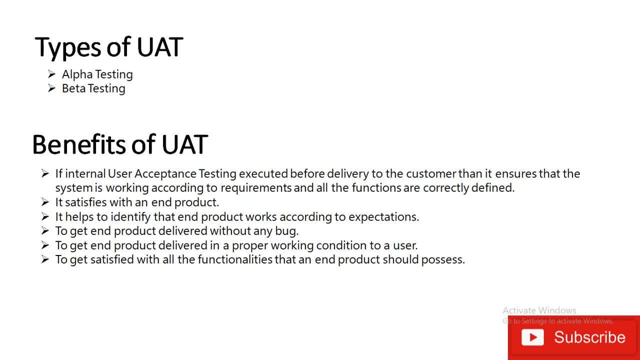 application, then there is a defect and that is not meeting to their expectation. so any functionality is missing and anything is not to the mark, to the application or to the requirement. that is a defect. for the uat team to get end product delivered without any bug is major or the 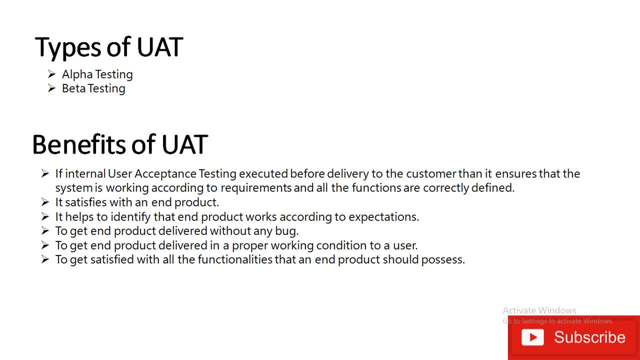 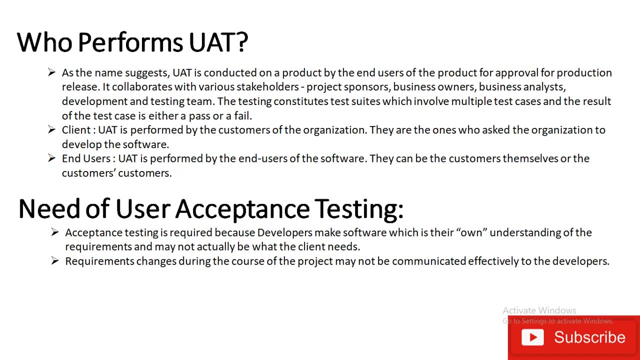 target of the uat team to get end product delivered in a proper working condition to user to get satisfied with all the functionality that an end product should possess. who will perform the uat testing is the major concern and when we are talking on the software testing, it always 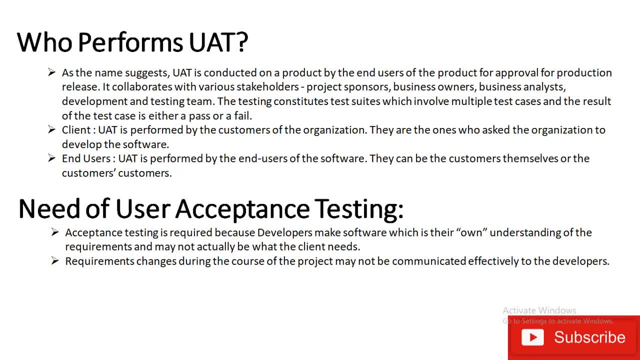 comes in my mind that in the complete phase of the development for that application, who will do that? the uat testing- as the name suggests, uat testing- is the uat testing. that is the uat testing. that is the uat testing. that is the uat is conducted on a product by the end user of the product for approval, for productions, release. 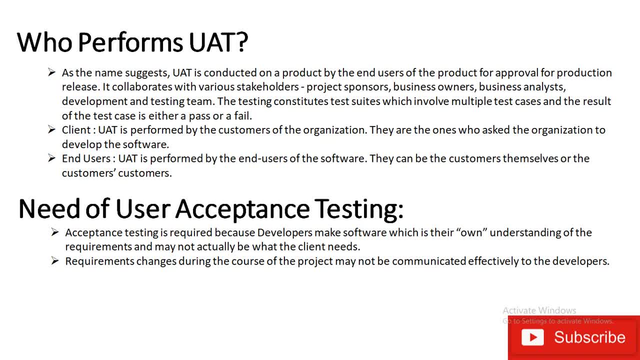 it collaborates with various stakeholders: project sponsor, business owner, business analyst, development and testing team. the testing constitutes test suits, which involves multiple test cases and the result of the test cases, either a pass or a fail. then the client uat is performed by the customer of the organization. 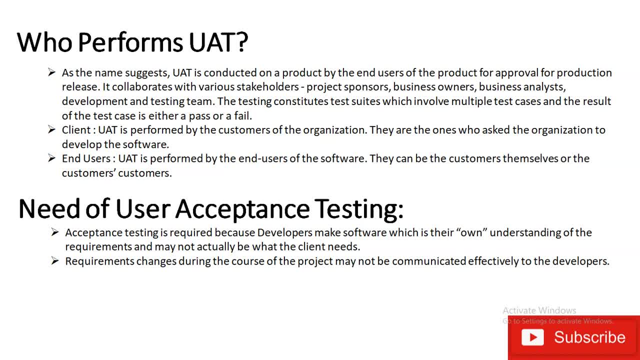 by the software user. they are the ones who ask the organization to develop the software end user. uat is performed by the end user. that is the part of beta testing and that time they will get beta testing release. they can be the customer themselves or the customer's customer. why we need? 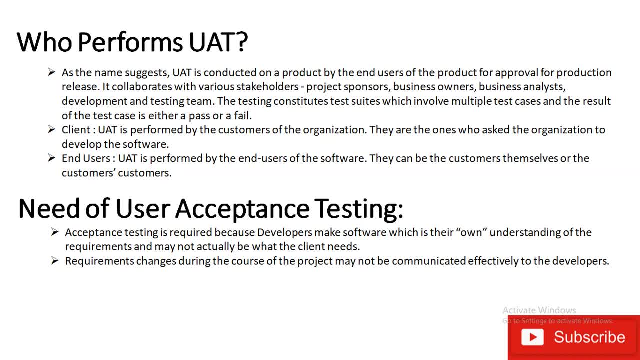 user acceptance testing in software testing phases or before delivering that product. acceptance testing is required because developers make software which is available to the customer for trial and which is either own understanding of the requirements and may not actually be what the client needs. requirement changes during the course of the project may not be communicated. 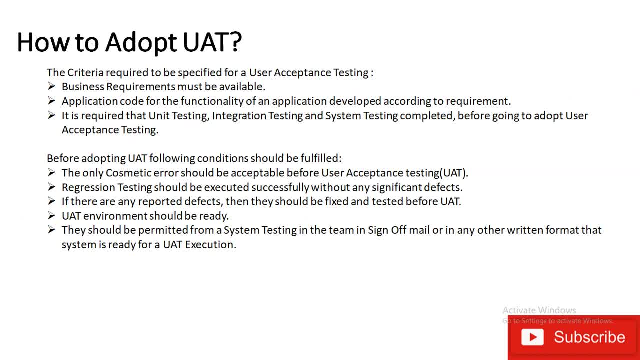 effectively to the developers. how to adopt uat testing is the main concern. while performing uad testing, the criteria required to be satisfied for a user acceptance testing business required must be available application code for a functionality of an application developed according to requirements. it is required that unit testing, integration testing and system testing completed. 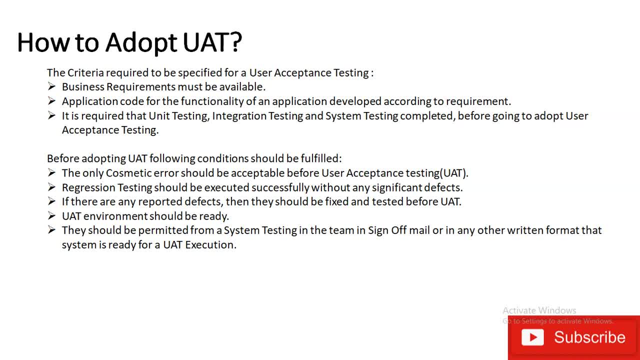 before going to adopt user acceptance testing. before adopting uat, following conditions should be fulfilled: the only cosmetic error should be acceptable before user acceptance testings. registration testing should be executed successfully without any significant defects. so what about the cosmetic errors? cosmetic error is a text issue. any of the blur images or anything related to ui part. 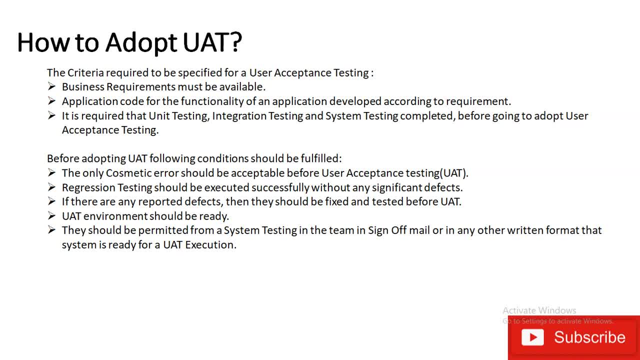 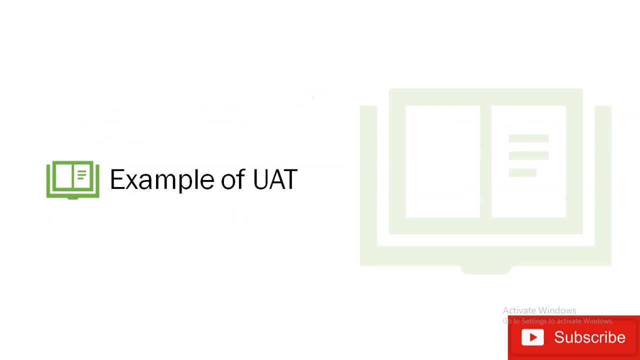 is a, basically a cosmetic error. if there are any reported defects, Ahmedім, give its a instead i. we sound doubts, i swap. give it a same, just like surat, save current pluginsva, eswat and amazing example. this time I'm taking one other example. let's take an example. 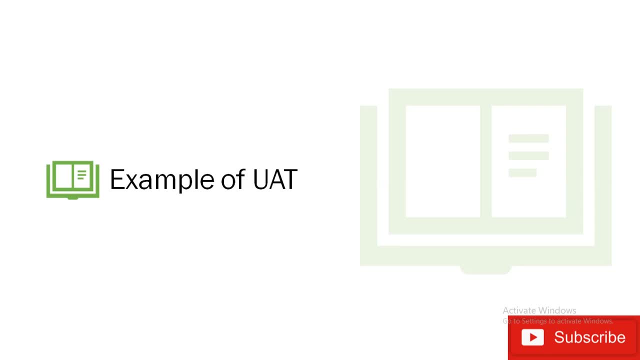 of any websites which are providing, or just take an example of UDI profile, so where we are creating our PF accounts, or, or we can call it. just take an example of Twitter. so Twitter is a web-based application and mobile application. both are available, so for testing both- the application in UAT, these applications. 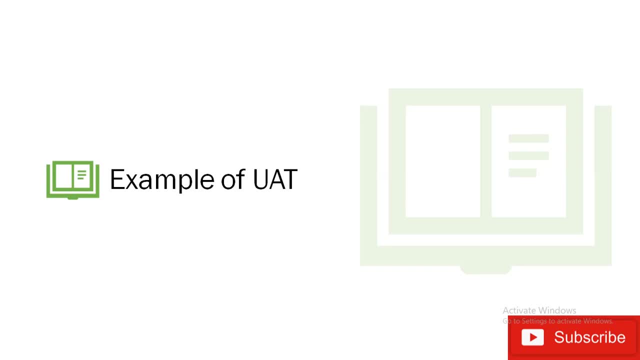 should be certified from the QA team. so in web-based application login should work properly. their functionality like tweet and other features should work according to their requirements. while posting that post should be visible depends on their privacy of the user who said that post should be visible to the user. post should be clear images. while uploading images should be.